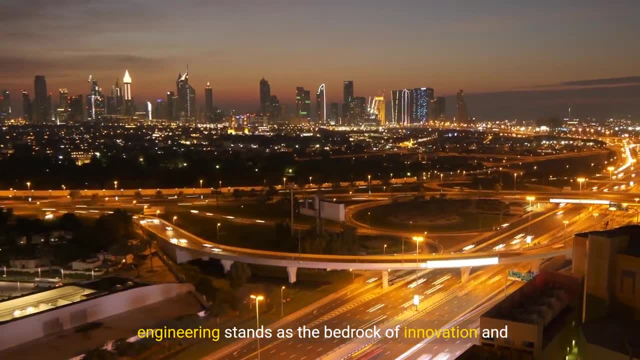 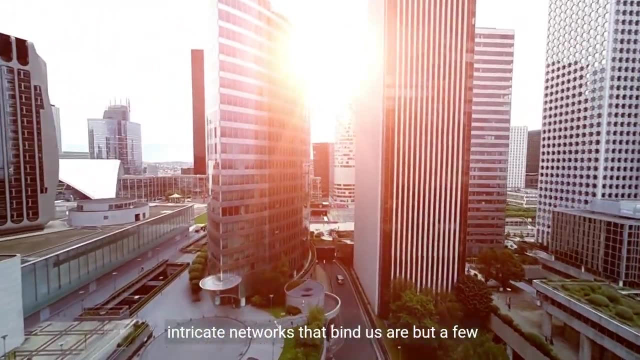 In today's exponentially evolving world, engineering stands as the bedrock of innovation and growth. Skyscrapers reaching for the heavens and the intricate networks that bind us are but a few examples of engineering marvels that shape our existence. These feats are not merely 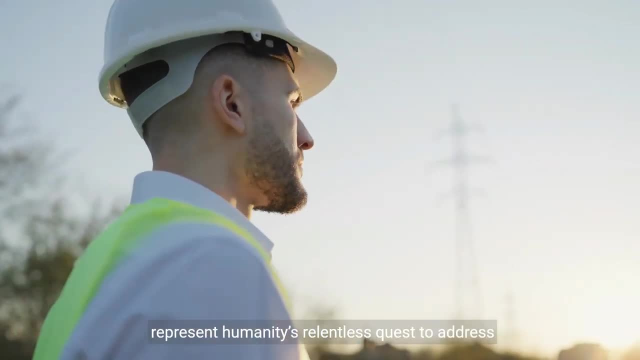 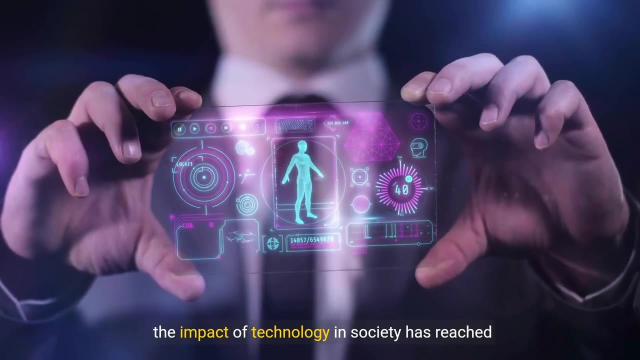 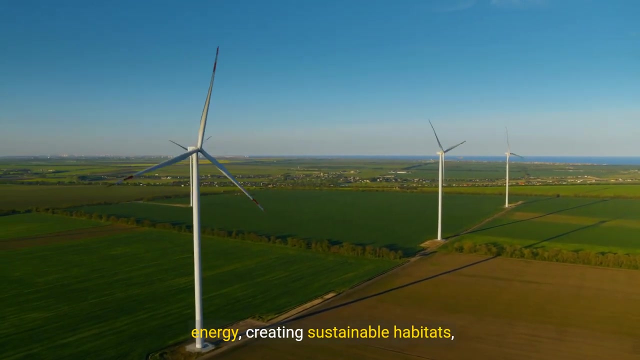 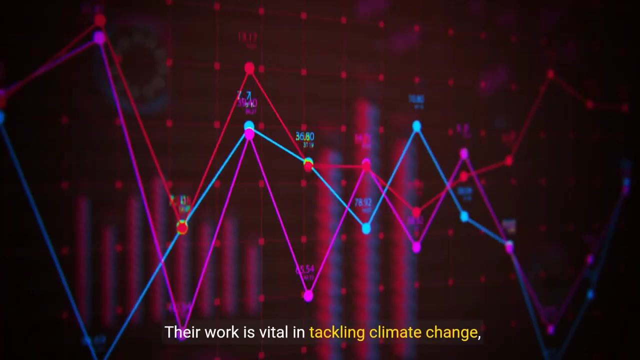 accomplishments, but represent humanity's relentless quest to address global challenges. At this pivotal moment in history, the impact of technology in society has reached unprecedented levels. Engineers worldwide are forging paths in renewable energy, creating sustainable habitats, pushing the boundaries of biomedical engineering and exploring the vastness of space. Their work is. 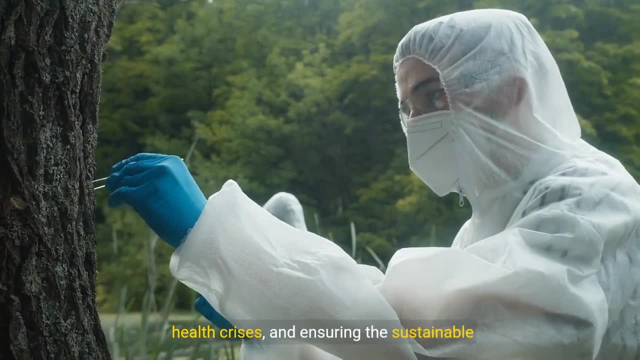 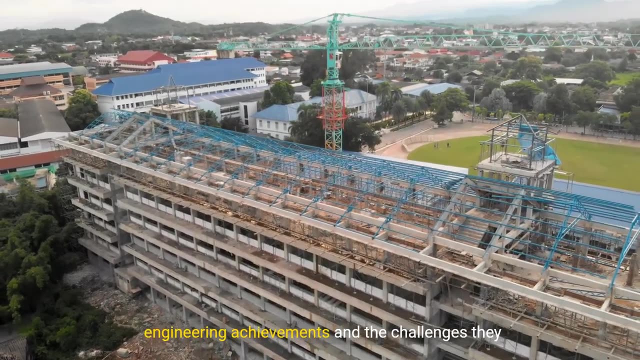 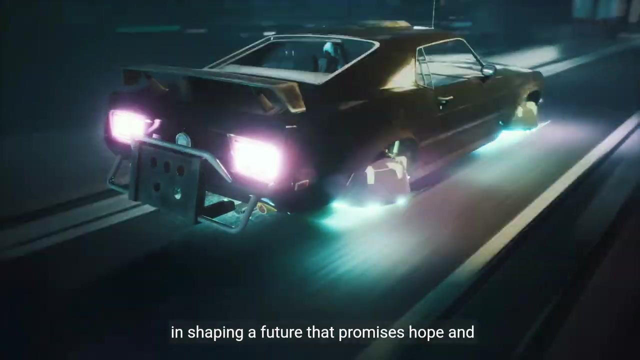 vital in tackling climate change, health crises and ensuring the sustainable stewardship of Earth's resources. Join us on a journey that showcases current engineering achievements and the challenges they aim to surmount. This expedition underlines the role of engineering in shaping a future that promises hope and innovation, guided by the principles of sustainability. advanced 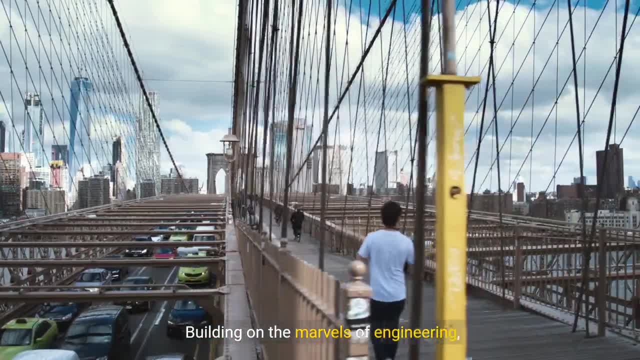 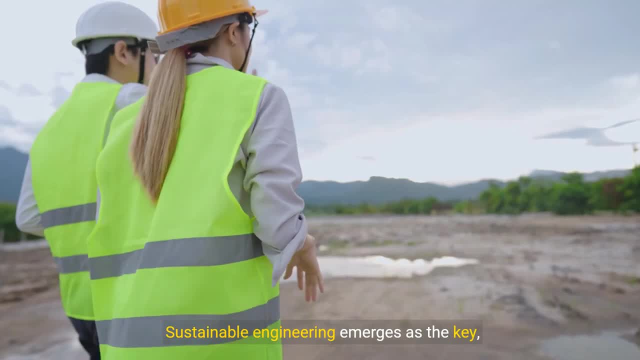 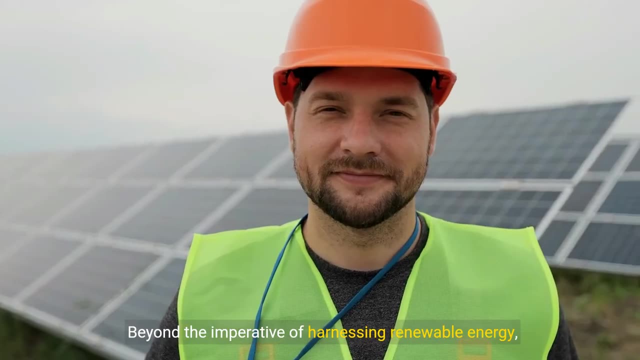 technology and space exploration. Building on the marvels of engineering, we turn towards a future where innovation intertwines seamlessly with environmental stewardship. Sustainable engineering emerges as the key propelling us towards a harmonious coexistence with our planet. Beyond the imperative of harnessing renewable energy, it encompasses the development of eco-friendly 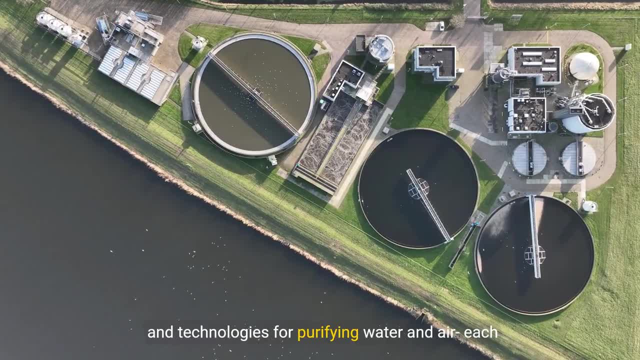 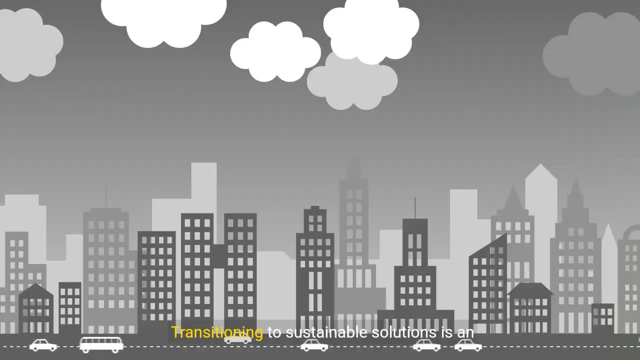 materials, construction practices and the development of new technologies. This is an opportunity for all of us to take a step back and look at the future ahead, Each breath and drop becoming a testament to our commitment to the Earth. Transitioning to sustainable solutions is an 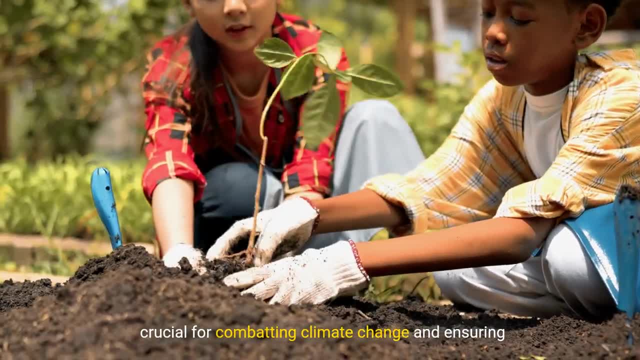 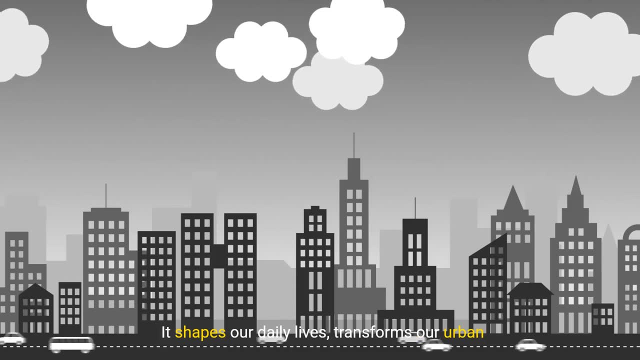 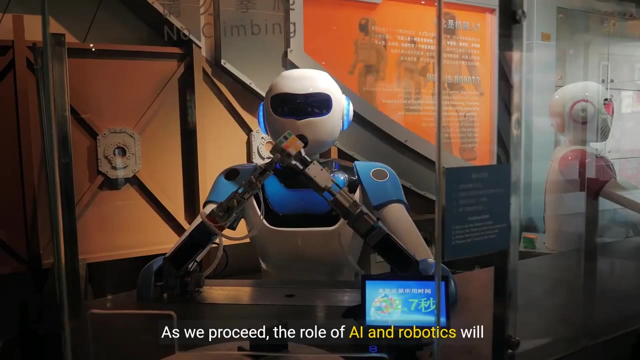 existential need, crucial for combating climate change and ensuring a habitable world for future generations. It shapes our daily lives, transforms our urban landscapes and purifies the air we breathe, forging a legacy of resilience and respect for nature As we proceed. the role of AI and 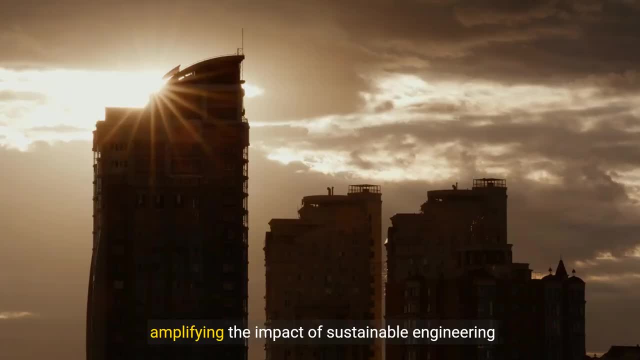 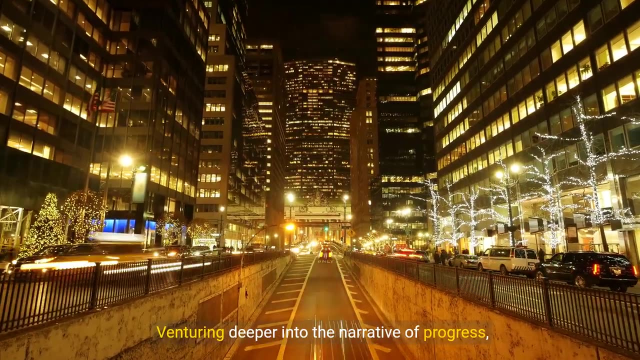 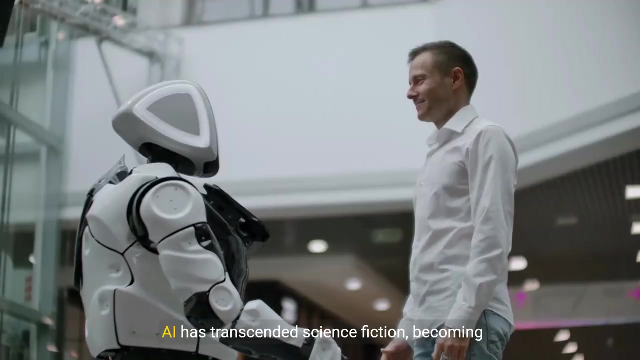 robotics will become evident, amplifying the impact of sustainable engineering and leading us to a greener, technology-driven tomorrow. Venturing deeper into the narrative of progress, the spotlight shifts to artificial intelligence and robotics, pivotal forces of the contemporary revolution. AI has transcended science fiction, becoming integral to our daily routines, while 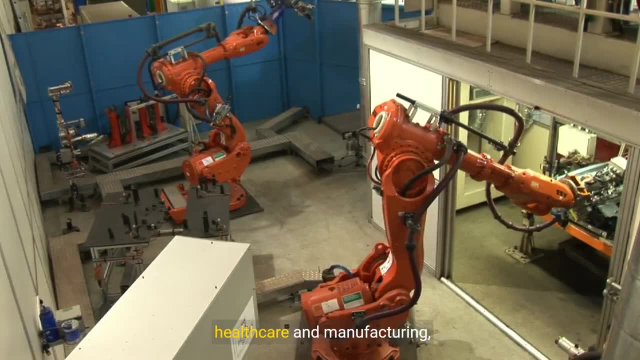 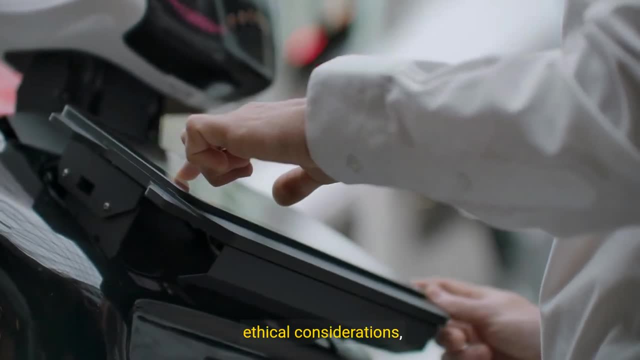 advanced robotics are making strides in healthcare and manufacturing, promising unmatched precision and customization. Yet AI is not the only technology that can transform our lives. It is the technology that can transform our lives. This technological leap beckons us to ponder ethical considerations, including privacy and employment implications, urging a balanced approach where 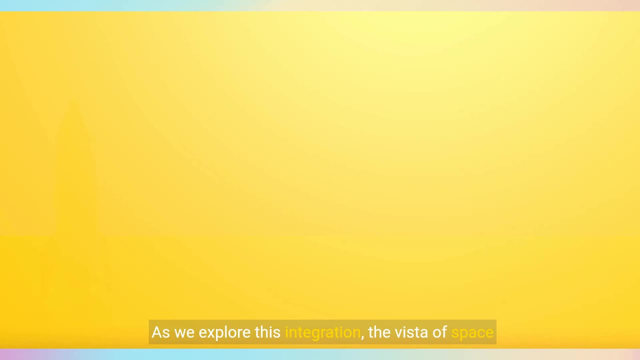 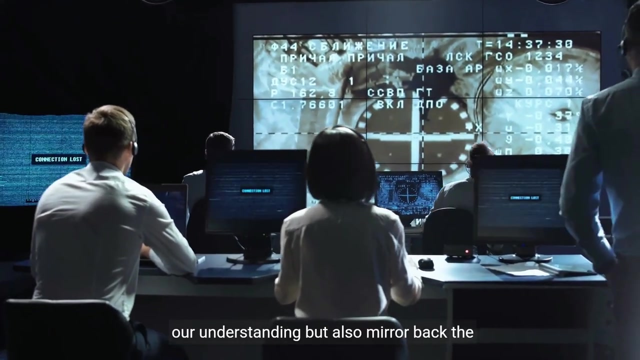 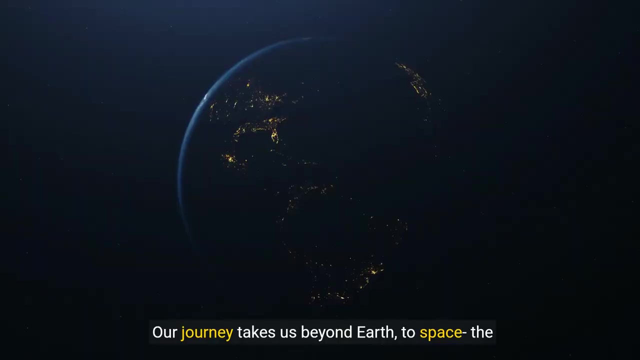 innovation aligns with our core values. As we explore this integration, the vista of space exploration awaits, revealing how our cosmic pursuits not only broaden our understanding, but also mirror back the ingenuity required to navigate our planet's pressing challenges. Our journey takes us beyond Earth to space, the ultimate frontier. 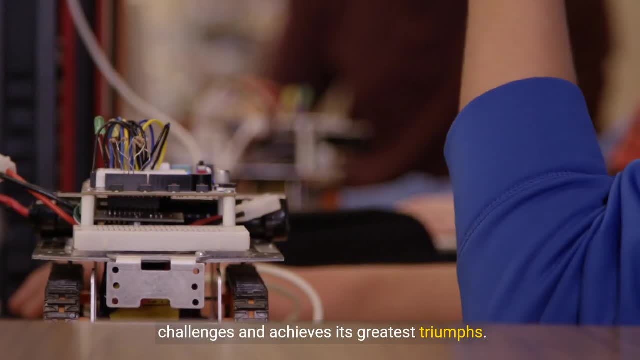 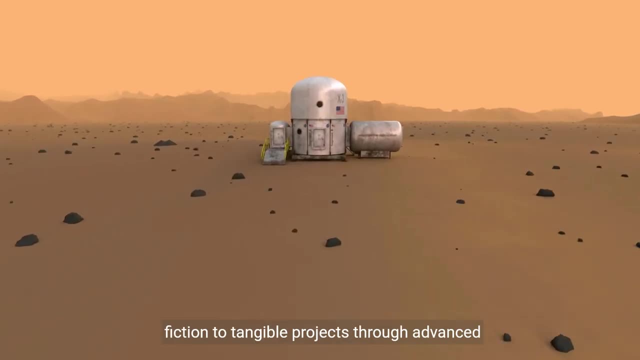 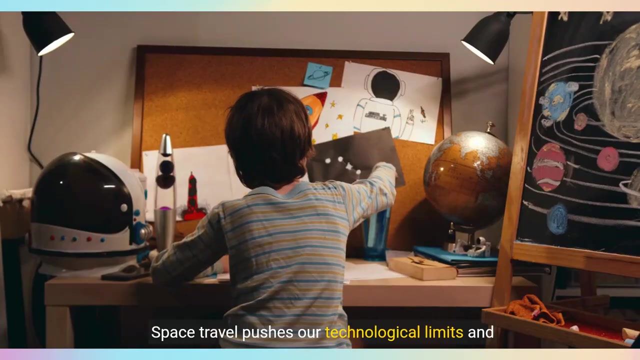 where engineering faces its most audacious challenges and achieves its greatest triumphs. The dream of Mars colonization transitions from fiction to tangible projects through advanced life support systems, habitation modules and strategies for sustainable resources. Space travel pushes our technological limits and fuels our imagination. 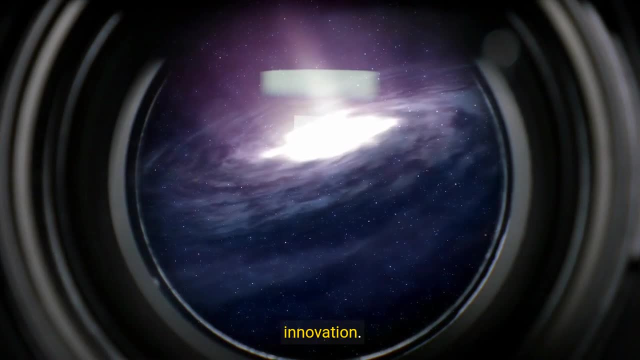 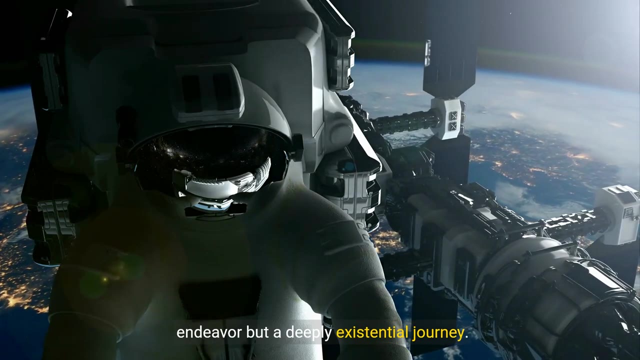 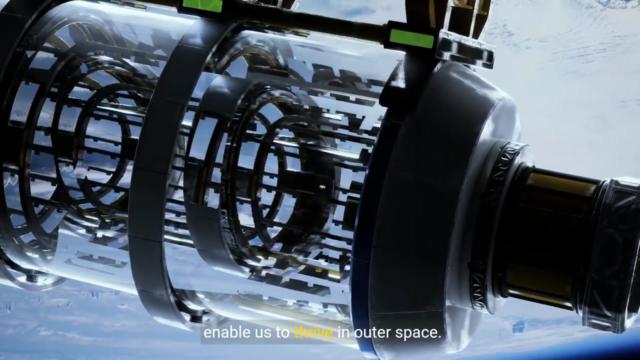 making the distant stars a little closer with each innovation. Space exploration epitomizes not just a technical endeavor but a deeply existential journey. As we aspire to venture beyond our home planet, engineers are the torchbearers confronting the unknown with solutions that could enable us to thrive in outer space. 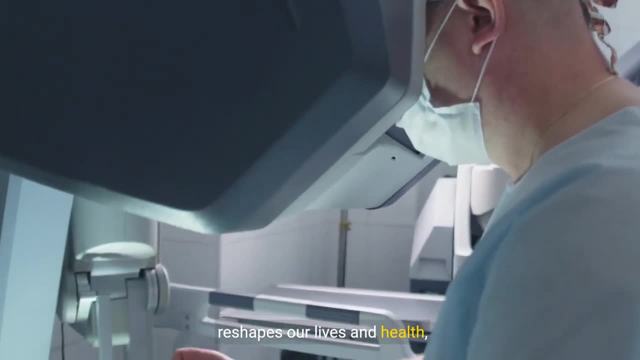 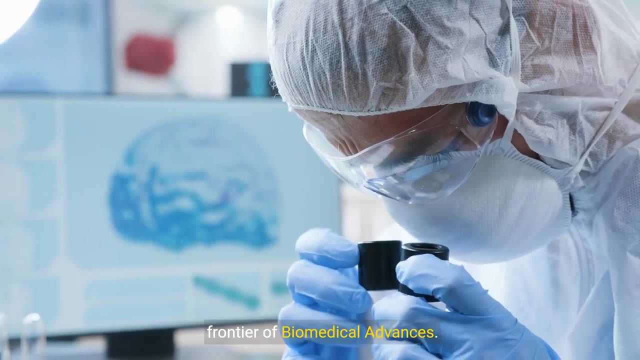 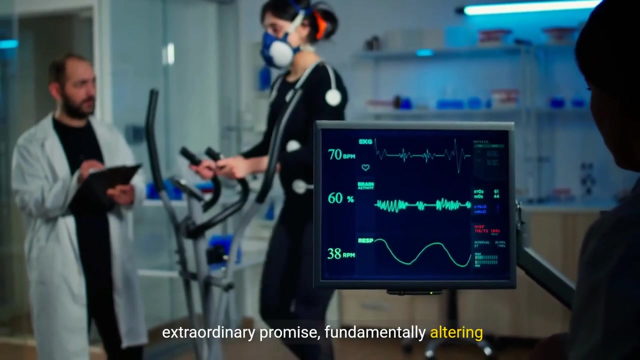 Here the narrative extends into how technology reshapes our lives and health, marking a new frontier of engineering potential. As our exploration progresses, we confront the vital frontier of biomedical advances. The path to engineering healthier lives unveils extraordinary promise, Fundamentally altering healthcare. 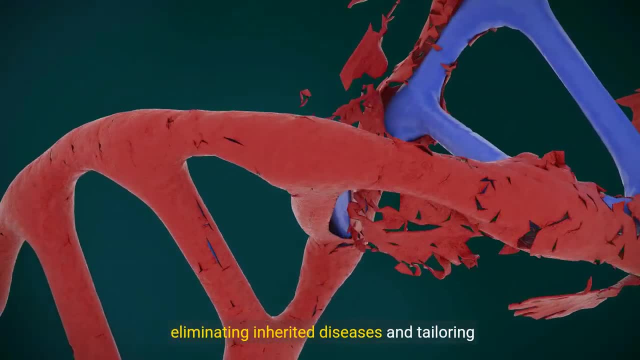 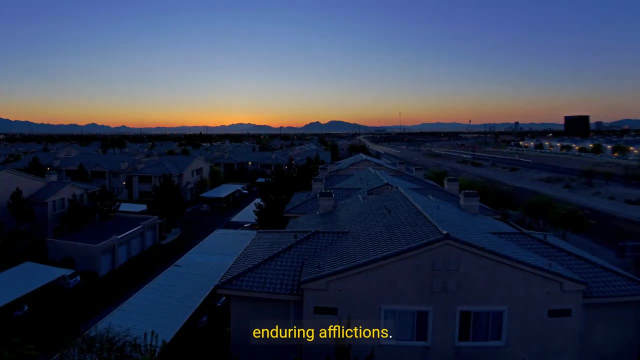 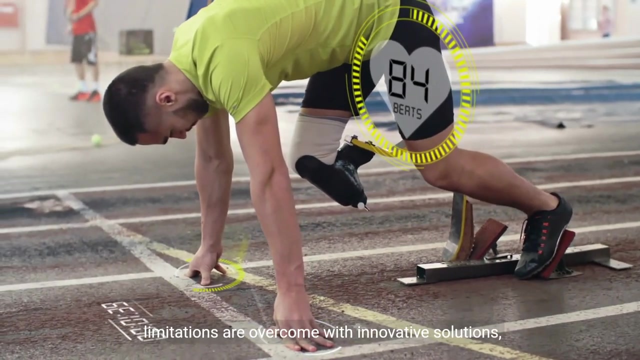 Genetic engineering stands on the brink of eliminating inherited diseases and tailoring treatments to individual genetic profiles, heralding a new chapter in our battle against enduring afflictions. Developments in prosthetics and organ printing are setting the stage for a future where physical limitations are overcome. 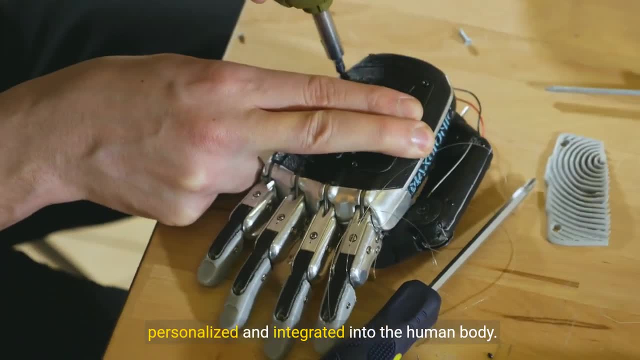 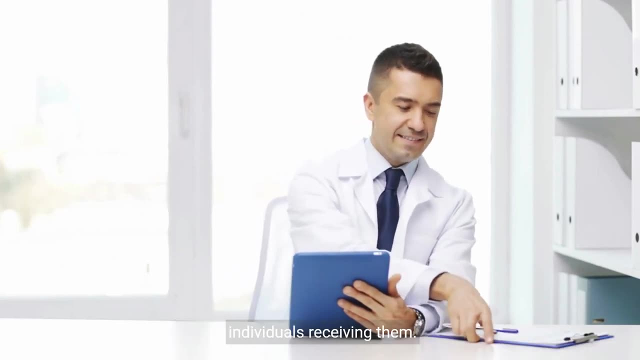 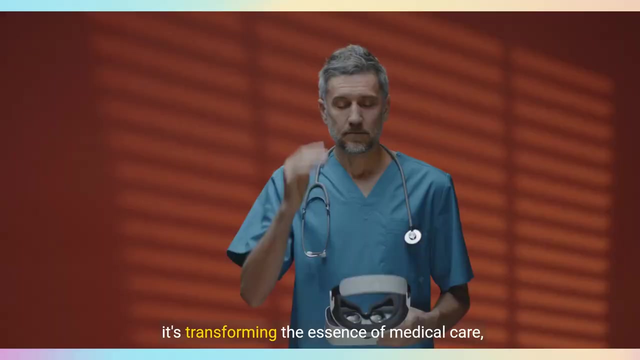 with innovative solutions personalized and integrated into the human body. Personalized medicine epitomizes this evolution, ensuring treatments are as unique as the individuals receiving them. This convergence of engineering and biomedicine is not simply about improving lives. It's transforming the essence of medical care. 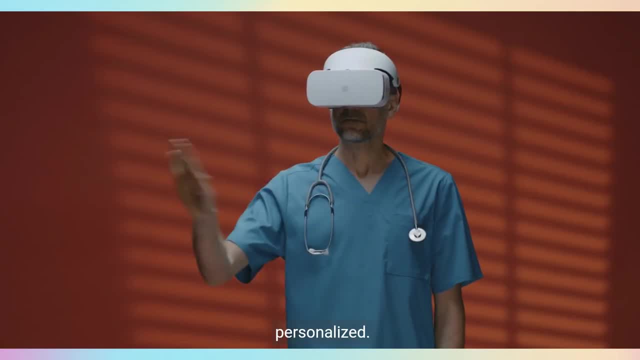 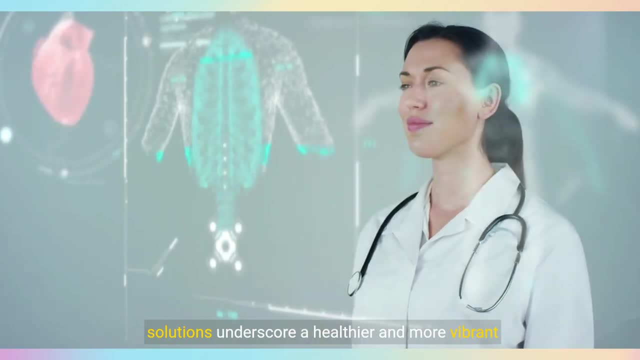 making it more effective, empathetic and personalized. It signals the dawn of a new era in healthcare, promising a future where personalized healthcare solutions underscore a healthier and more vibrant humanity.